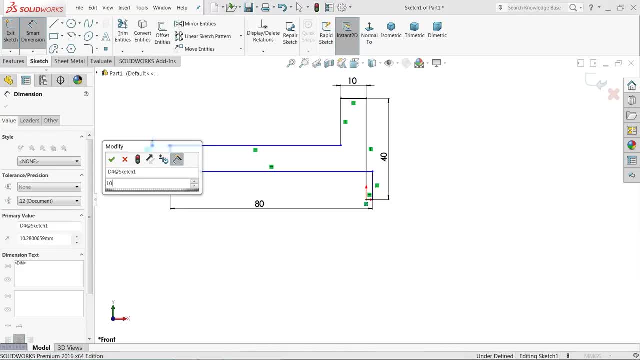 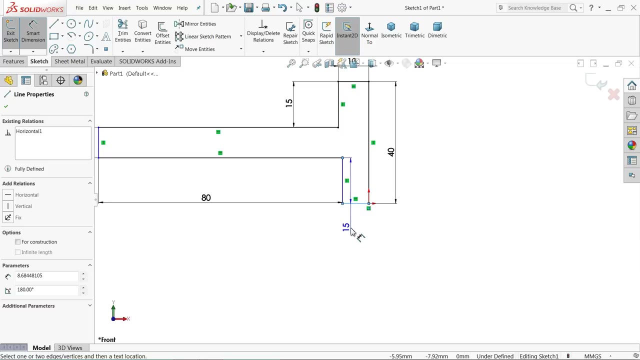 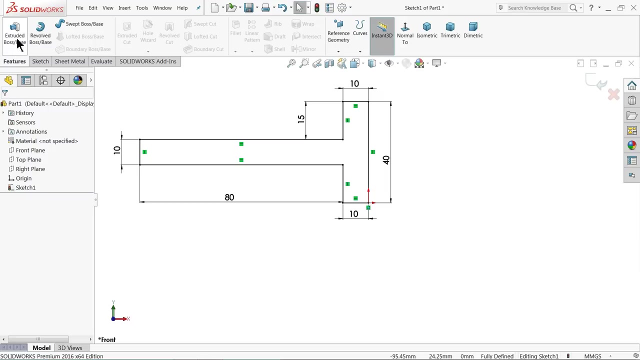 10 mm. Even this also. keep 10 mm, 15 mm. Now just this one, drag inside And keep this one 10 mm. I think some points selected here, Or even you, can make the relation equal. Now extrude it. Extrude upto 20 mm. 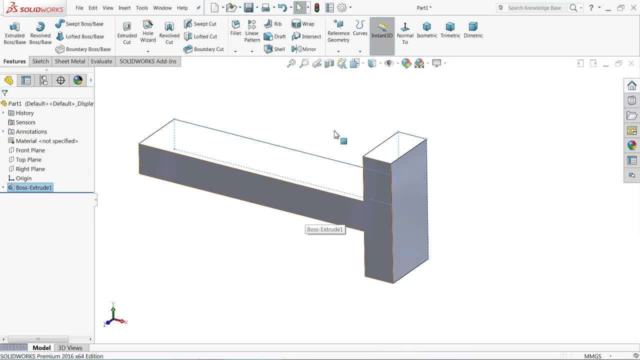 Now, here we will. We will see the stress and deformation in this structure, How it will deform, How it will strain. So first we need to go to solid work simulation. How you will go to solid work simulation. Solid work simulation either comes here or either comes in your normal system. 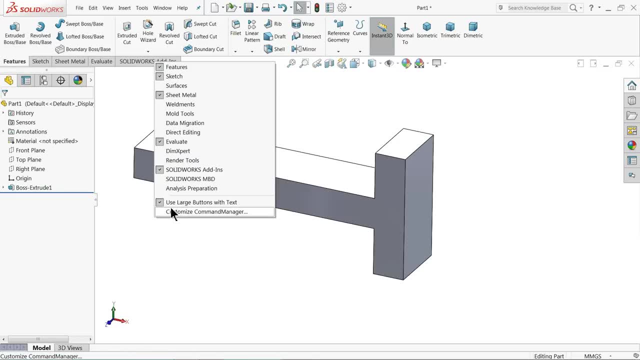 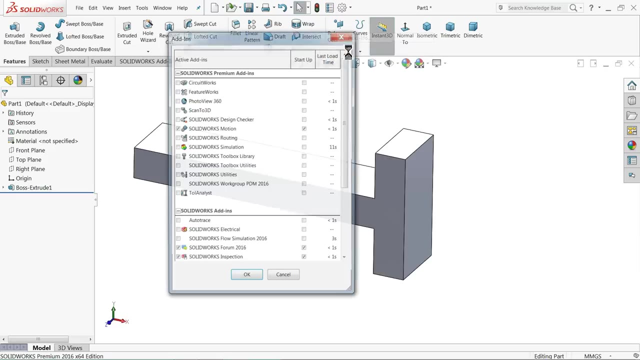 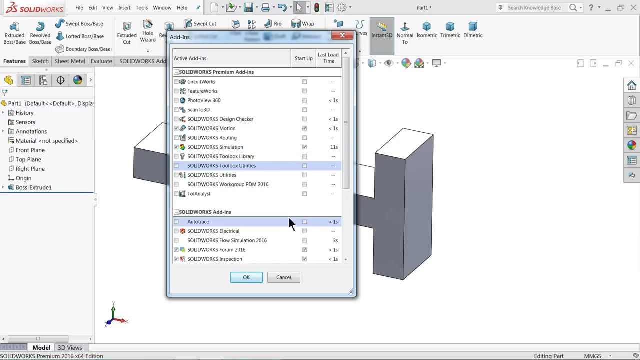 your command manager. Just right click on command manager and here should be simulation. but it is not here. So do one thing: Just go to here option, Click on this window, Just drop down this window, Select add-ins. Once you go to add-ins, you will find here SOLIDWORKS simulation. Just click check box both side. OK. 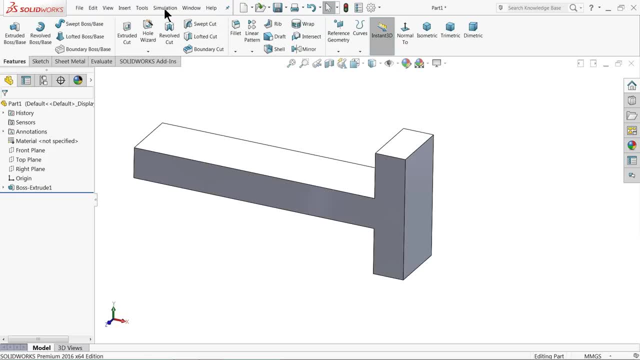 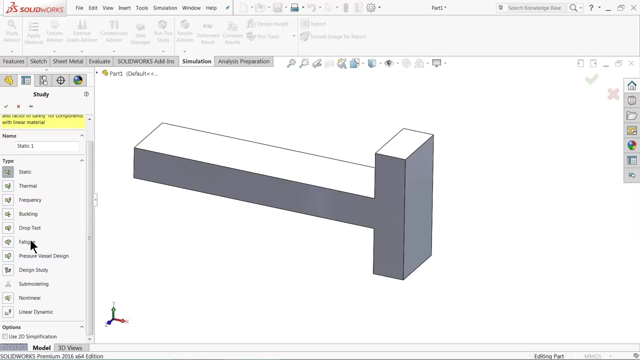 Now here you can see in your window minus, see simulation added here, and even in your command manager the simulation added here. Now, just it will ask you: study advisor or new study. So we are going to make new study Now. these are the different kinds of study or methods of test, like thermal frequency, buckling, drop test. There are many. We will learn each and every, everything, one by one. So do one thing. 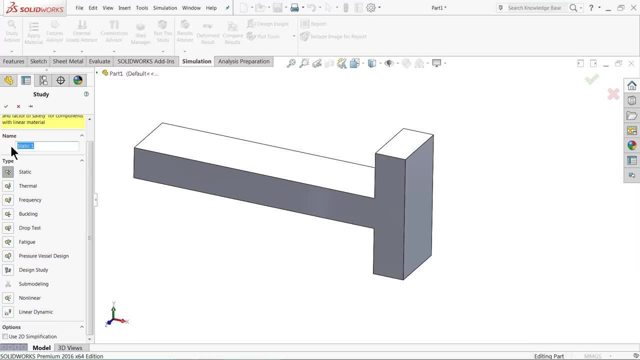 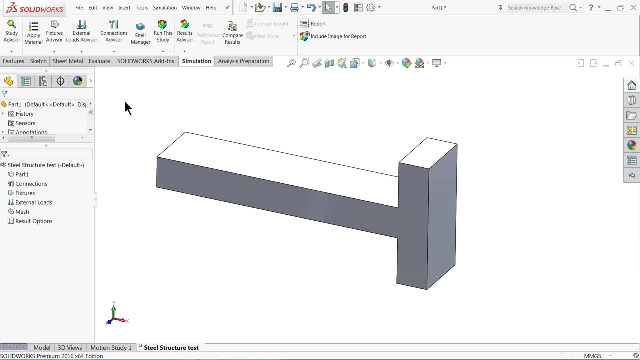 So let's do static test. You can give any name, It's up to you: Steel structure test. OK, Now you enter into the SOLIDWORKS simulation window. Now these are the little formalities. you have to do it First, select the part and you have to apply the material. Which kind of material is this? 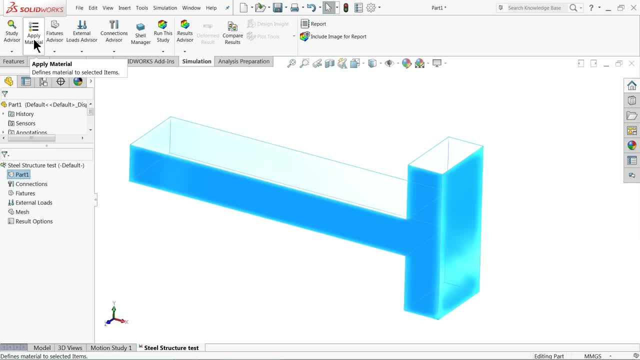 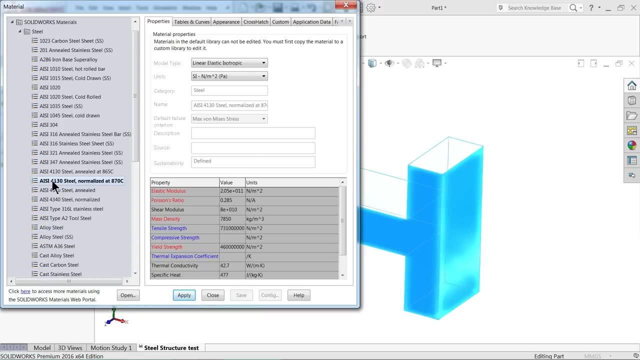 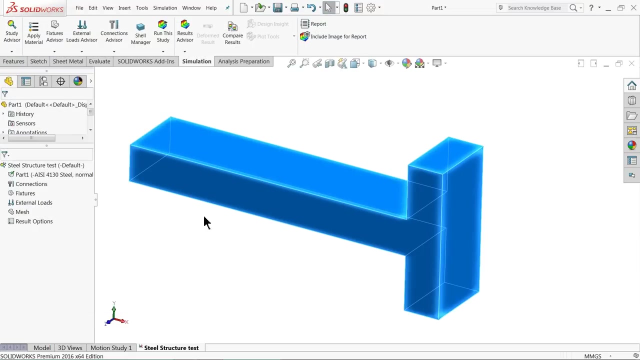 So here on top left corner you will see here apply materials. So any material we can apply here, like anything steel normalize at, apply Close. Now here we applied the steel to this body. Now the second stage is connection. It is not required Fixture, Fixture advisor. So you need to fix the geometry. 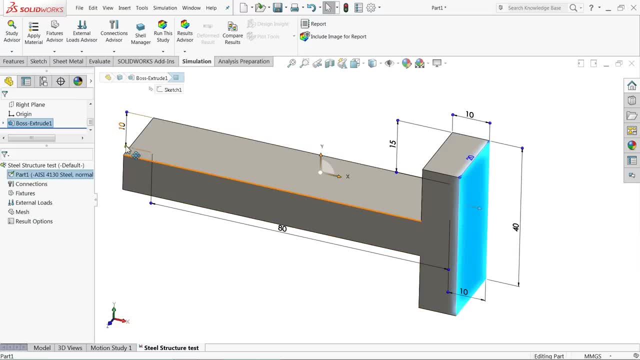 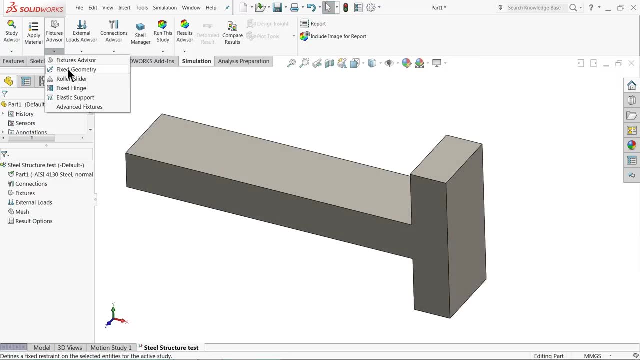 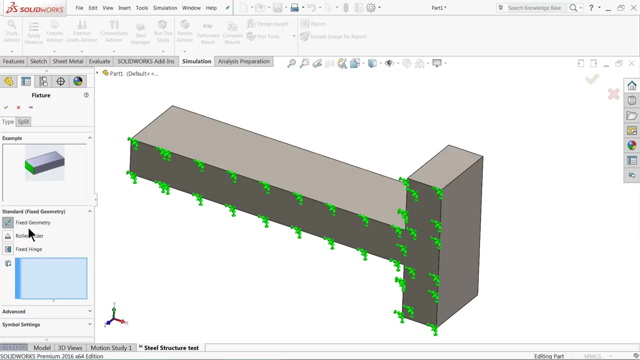 From any one place, Either from backside or anywhere. Then only we can find out the, we can apply the force and we will see how it behaves. So fix the geometry. We will fix the geometry from any one places. You will see there are three types of fixture: Fixed geometry- You can see in your left hand side, See roller- or slider fixture- It will slide along with the body- And fixed hinges. This is also a kind of, But we will try here. 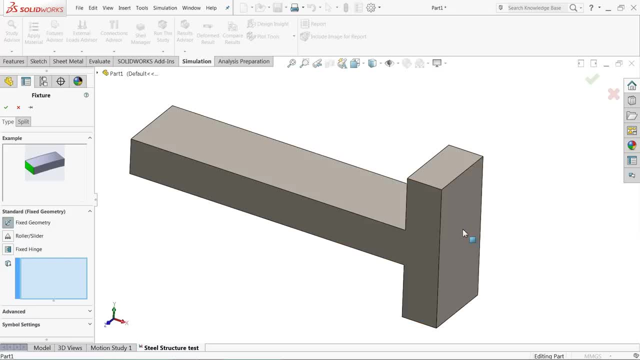 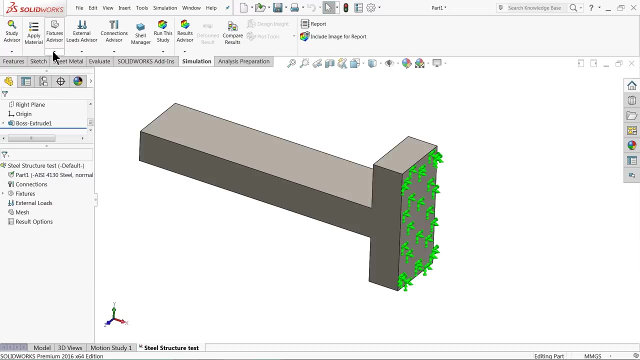 Fixed geometry. Let's fix this one Now, this right hand side wall we fix, So it will not. The body will move along this one, But this will not move. OK, Now, once you fix this one, Now we will apply a force. So, just next to the fixture advisor you will see external load advisor- External load. You can click from here or you can right click and apply from here. So let's see how it behaves. 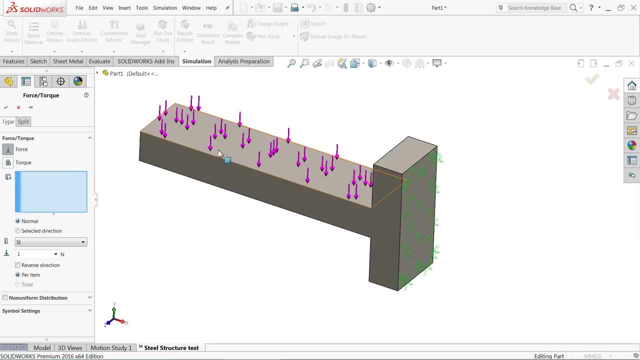 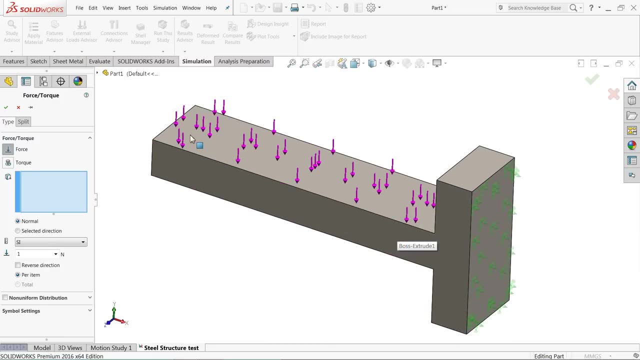 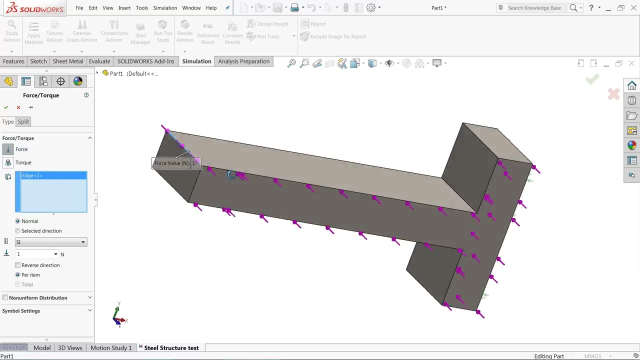 apply force. now see, you can apply force anywhere, but we will apply from top top direction so it will easily identify or study the behavior. so I'll choose this line because I am going to apply the force in this line so you can see. once you apply the force in this line, you can see the direction of arrow, the force. 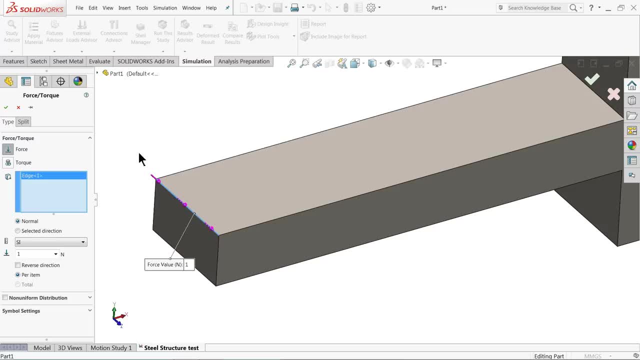 going toward this direction, but we want to. it should go a downward direction. so here, one option after normal. you will see: select selected direction. click on selected direction. now click on. once you select the click selected direction, you know you can select. let's say, I'll choose this vertical line, so see arrow. 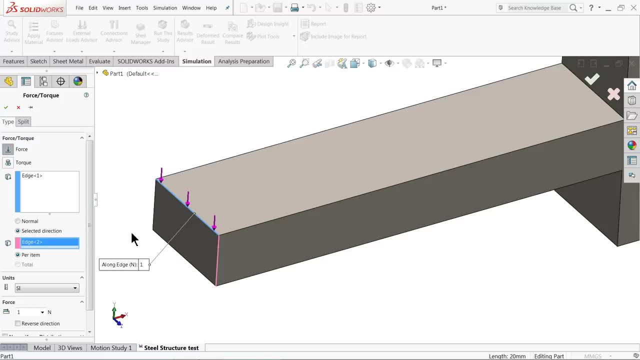 goes down, that means the force going to apply on downward direction. now, here I will apply the pressure or force, anything. I'll apply 200 Newton and we will see how it will impact on our steel structure. select- okay, now we fixed our geometry from one side and apply the force, so let's select the. 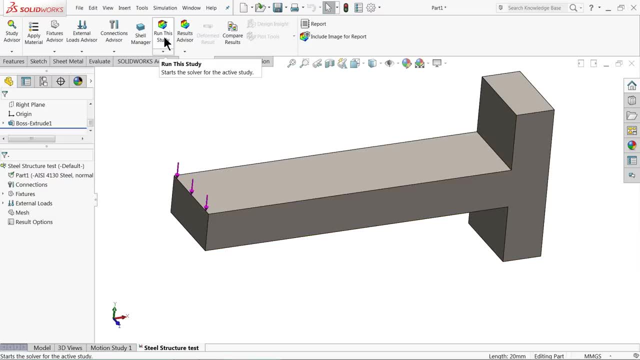 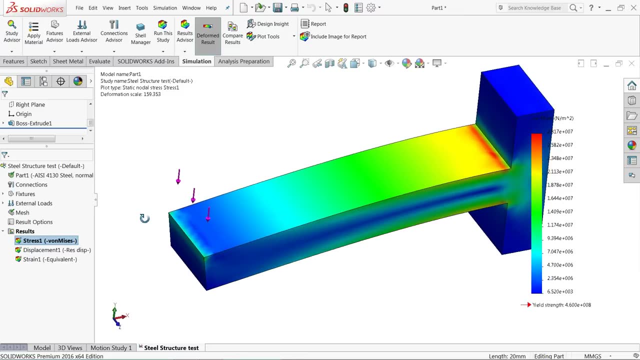 run this study, click. run this study. it's calculating. now see our steel structure. bend from where we applied the structure and you will see in your right corner a red mark. red mark means stress. the more stress is here it. if the pressure will be less, the stress will be more and it. 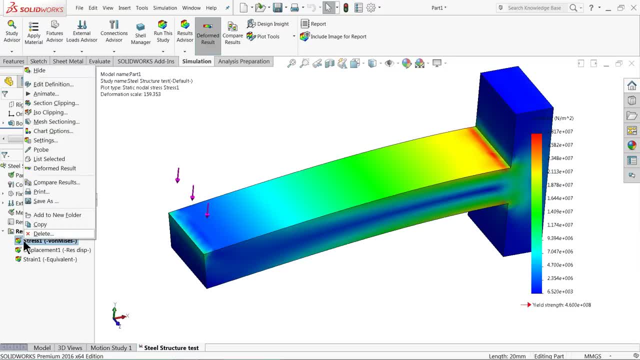 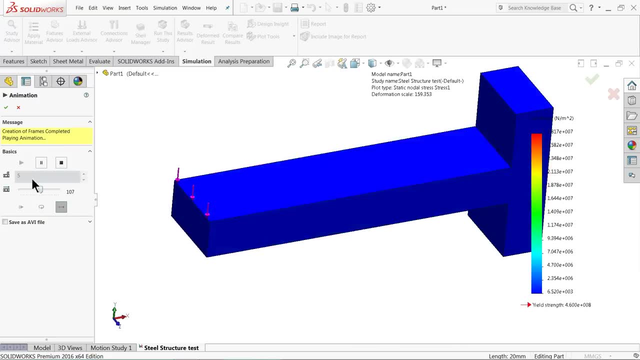 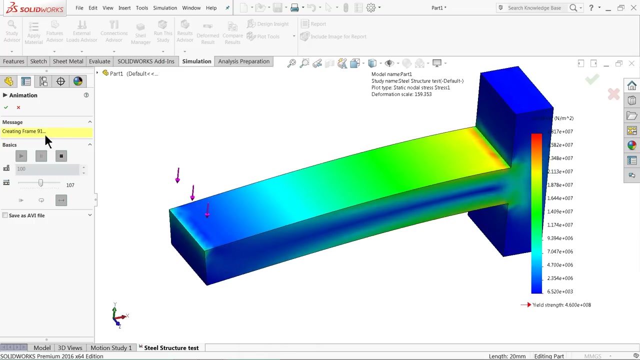 Y through 0on. attack range is 1966 specters. before running operation: See creating frame. Now, once we will increase this one, it will calculate and it will go faster. Now you can see if it is going down. the pressure applies. it goes down. At the corner you will see the red mark. This is the stress. 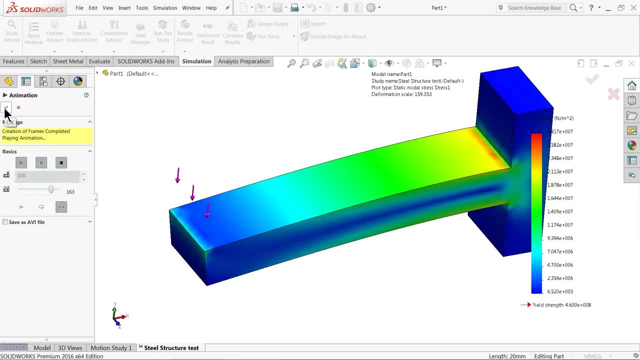 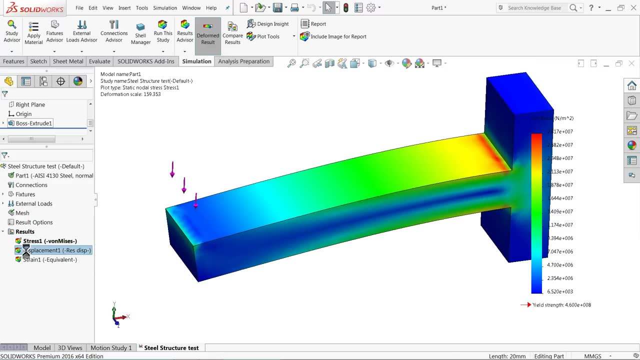 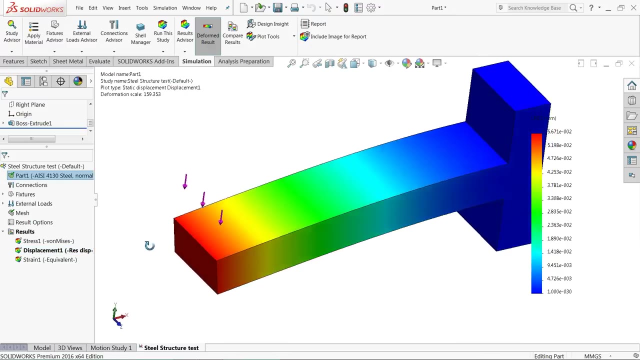 Now select here, apply. Now you can see the displacement. Now select on the double click on displacement. Now see the more displacement you will see in this corner area. See, this is the displacement of body. So the our force is much required. Force is greater than the steel structure. 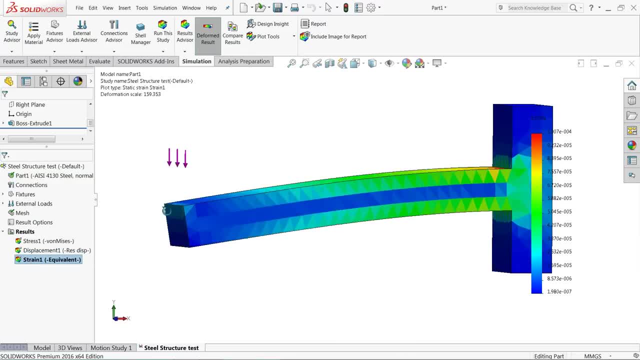 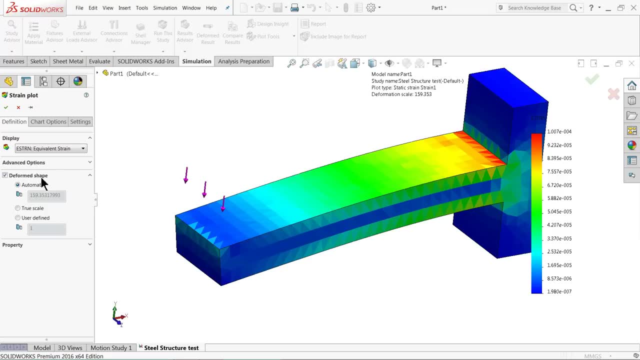 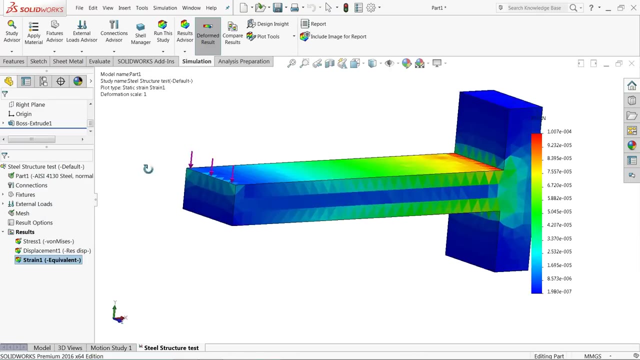 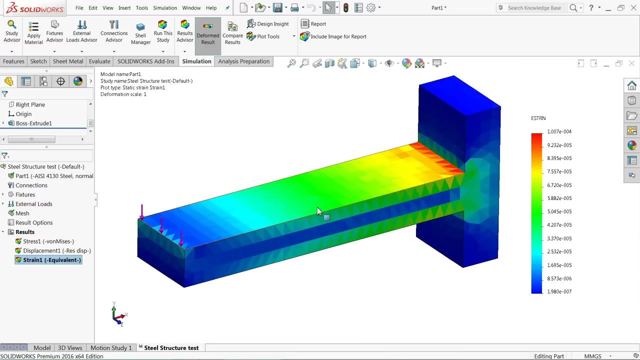 Now let's double click on the steel structure. Now let's double click on strain. Now we will force it and regain original shape. So right click, edit definition. Now see deformation shape. It is done by automatically. Let's choose true scale, Apply. Now it is: regain its own position. So this is the simple study of steel structure: How you will apply a force on any structure and you will see the deformation in any structure. I hope you like this tutorial. Don't forget to share and like our video.